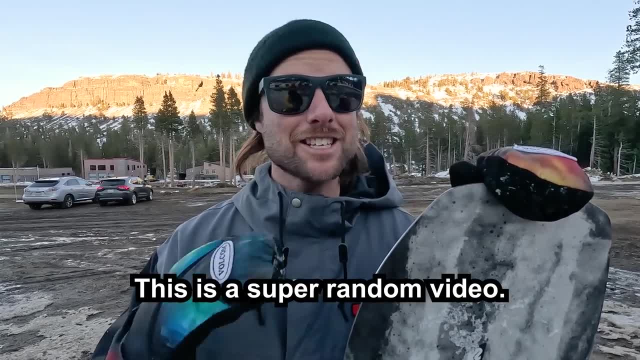 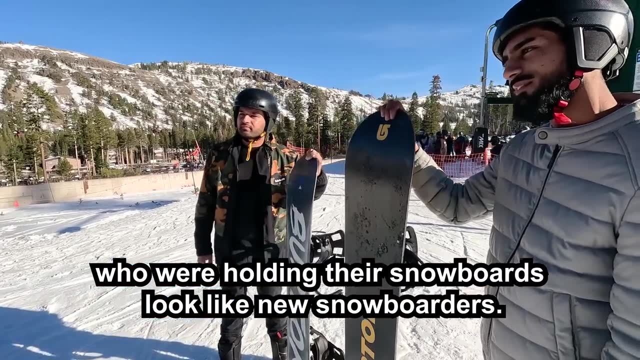 Yo, what's up everyone? This is a super random video. So I was in the lift line and I saw these two guys who were holding their snowboards look like new snowboarders. So this video is about teaching two strangers how to snowboard. Do you guys know which foot is more dominant? 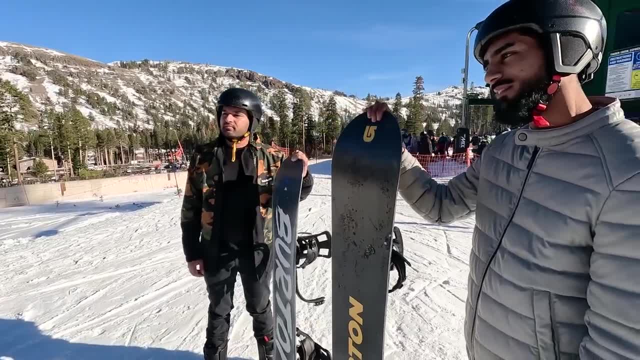 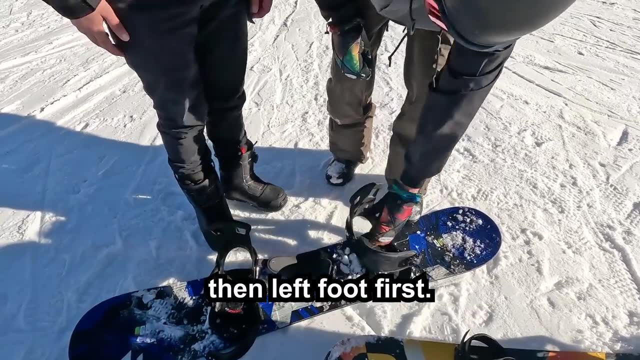 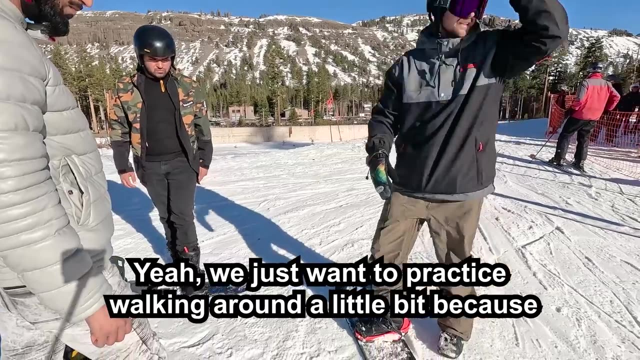 So if you're like kick a soccer ball, I'll go with the left, So strap in whichever one you guys think is your front foot. So for you, if your left foot is more dominant, then left foot first. So yeah, we just want to practice walking around a little bit, because so that 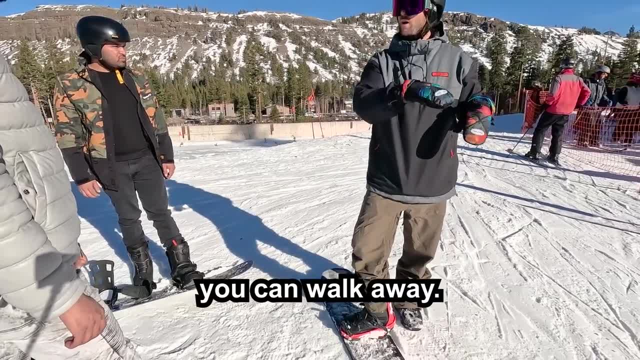 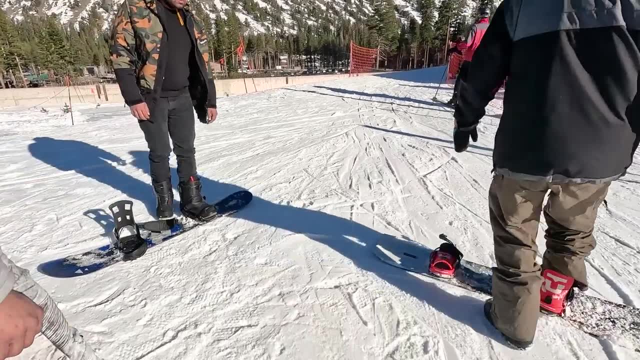 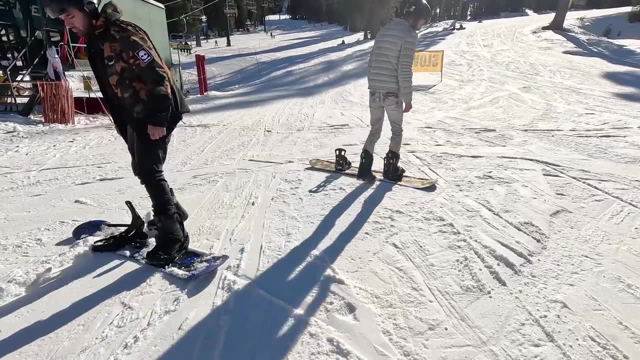 we can walk to the chair, and then, when you get off the chair too, you just have to like, walk away, And the easiest way to walk is to have your free foot behind, Push your board along And try to keep most of your weight on this foot. It's like skating. I never skated. 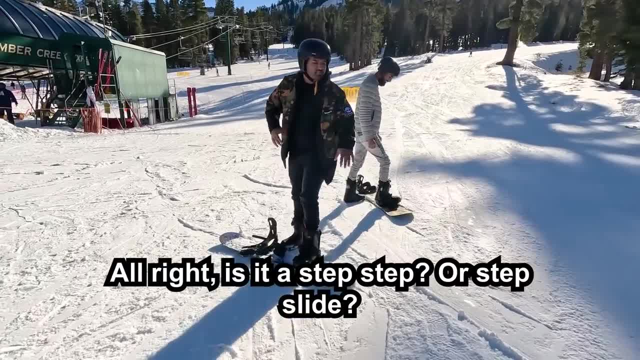 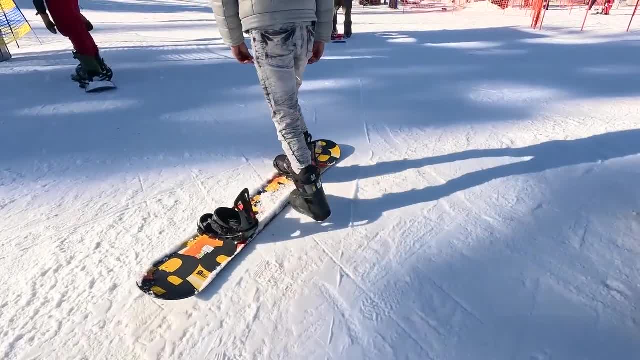 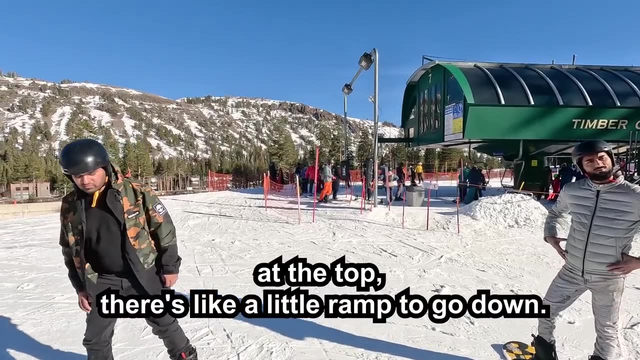 before either. All right, so is it a step step or a step slide, one Little steps to start. So this is called skating. It's just pushing with one foot is called skating. So when you go to get off the chair at the top there's like a little. 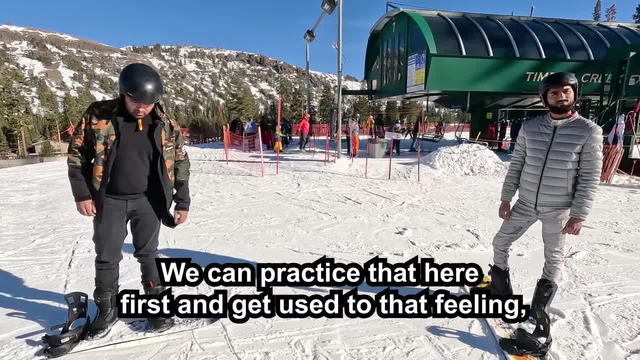 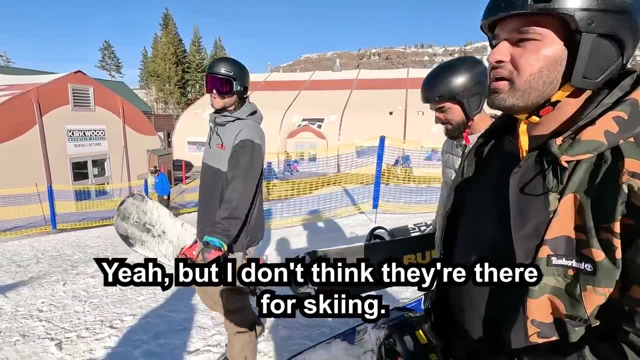 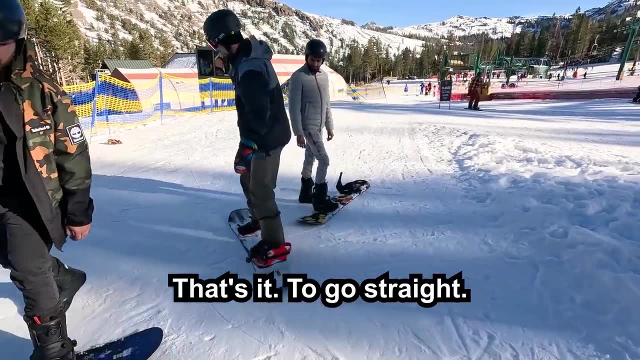 ramp to go down, So we can like practice that here first and get used to that feeling. I guess there's some pretty big mountains in Pakistan, right Yeah, but I don't think they're for skiing. Okay, They're just rough mountains, That's it. You go straight and then you stop and you just like drag your foot. 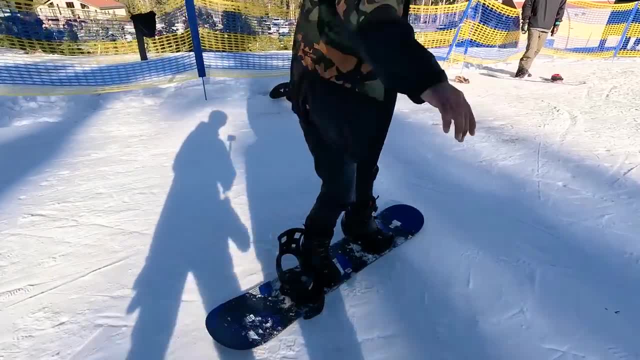 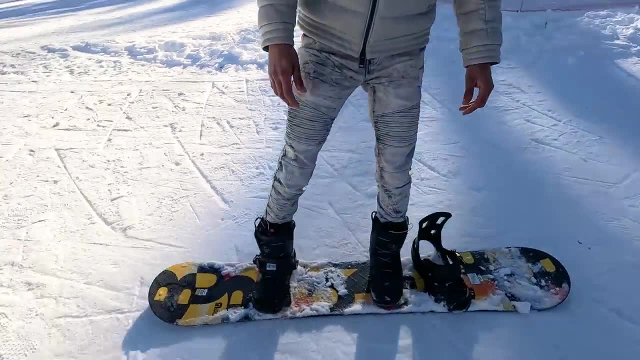 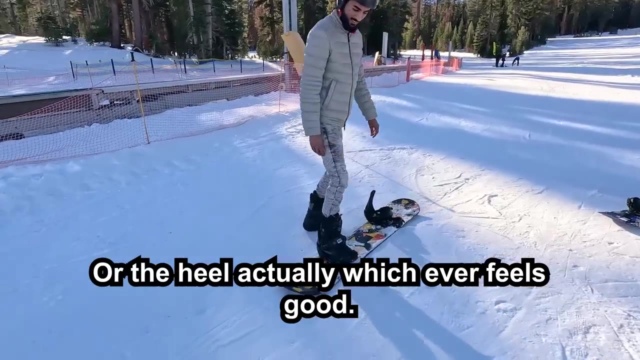 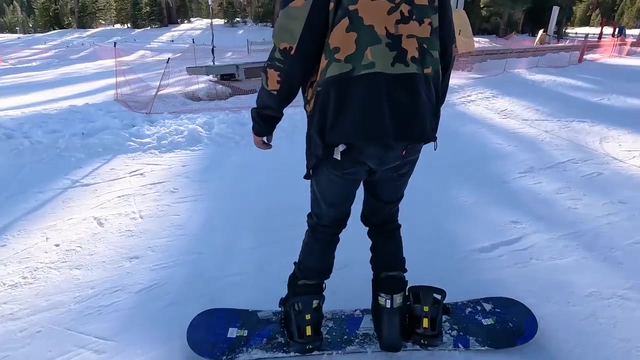 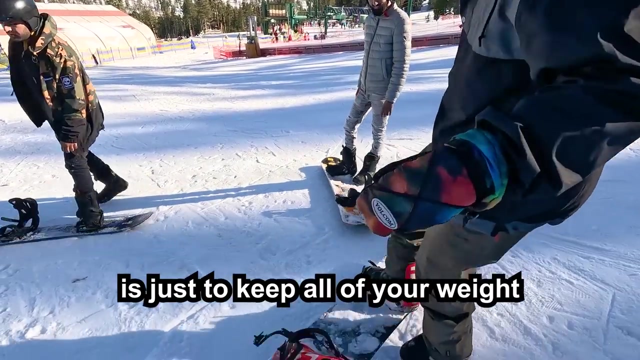 Yep, Straight, and then you just drag your toe, Boom, That's it. And then you drag your toe And then the heel, actually Whichever feels good, Perfect, Good try, dude. An easy way to be in control of your snowboard is just to keep all of your weight. 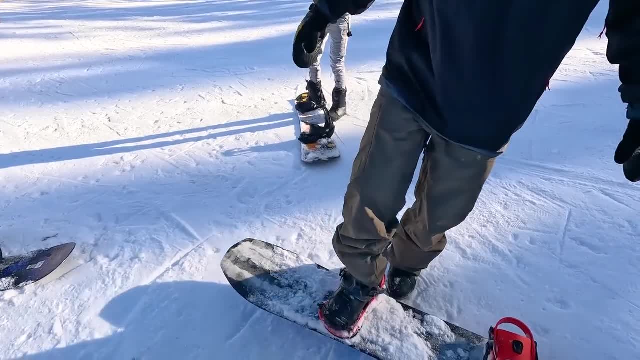 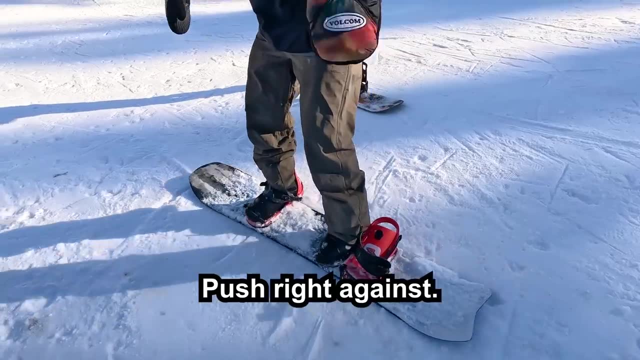 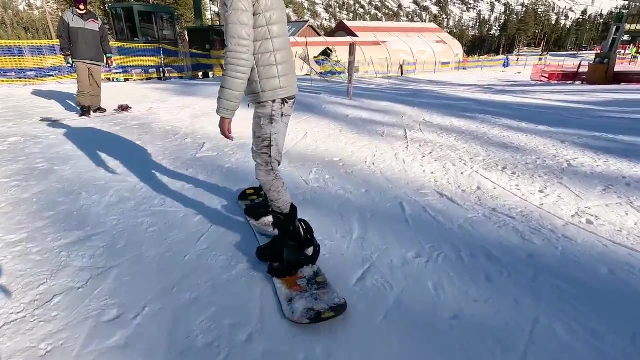 on your free foot, and then you can like move this however you like. A good way to keep your foot on the board, too, is to push your foot against the binding at the back. So push right against. Oh, perfect, perfect, That's it. 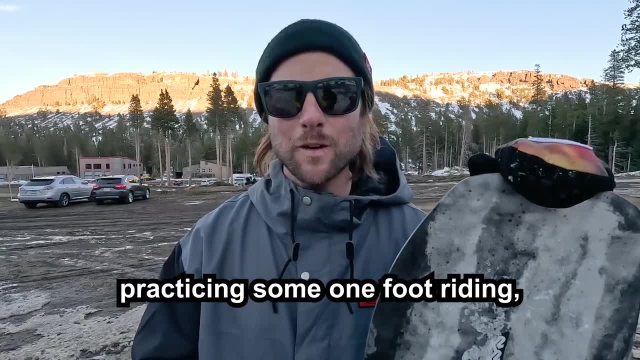 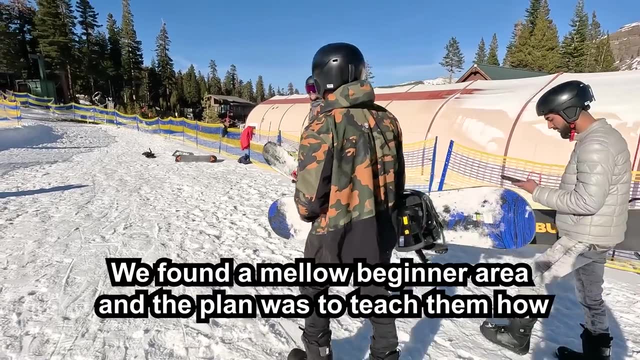 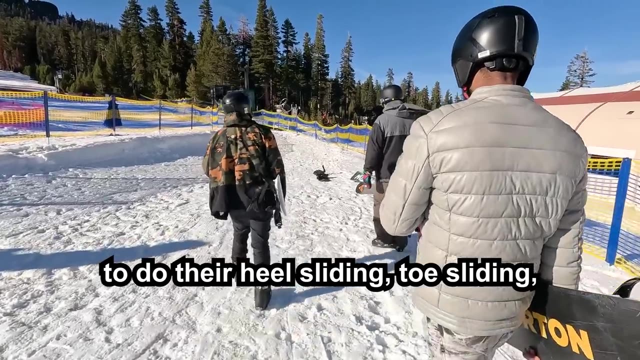 So, after figuring out which one was their front foot, practicing some one foot riding, I was thinking, instead of going to the chairlift straight away, should probably take them to a mellow area. So we found a mellow beginner area and the plan was to teach them how to do their heel sliding, toe sliding and maybe even get one or two turns going. 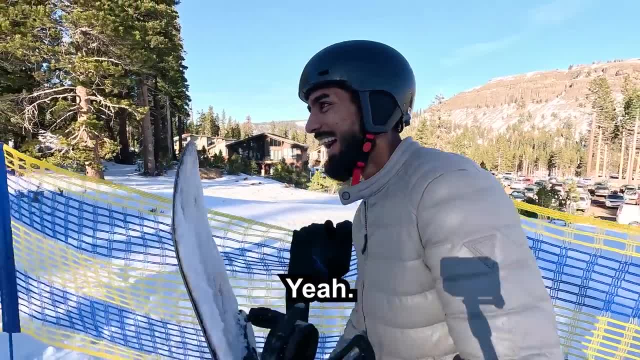 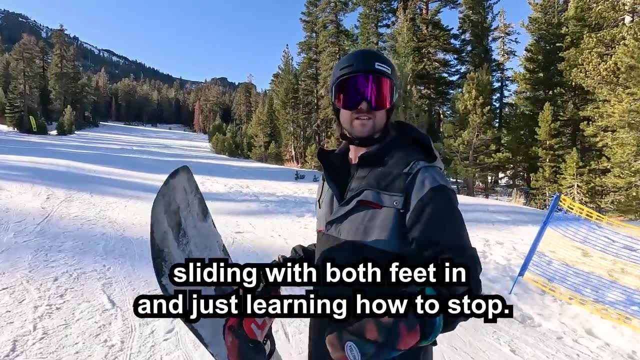 What's your confidence level? Oh, so like 10.. Gotta be confident, Yeah. so we do this practice up here, doing like uh, sliding with both feet in and just learning how to stop Z. what's your confidence level? Oh, still 10, even though I'm 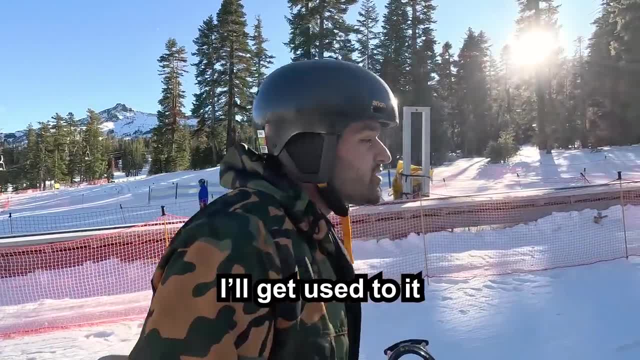 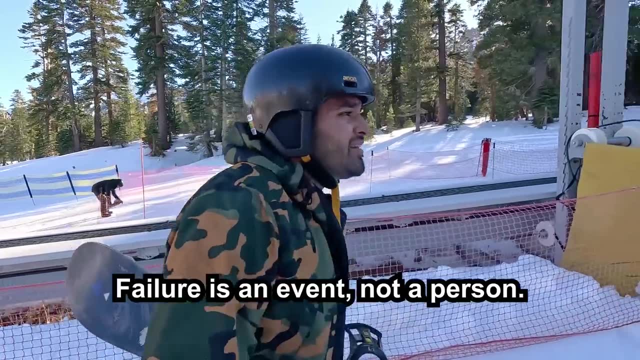 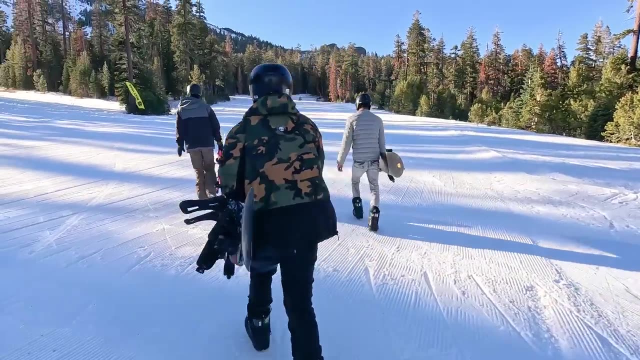 failing, But eventually- I'm a guy who's used to it- You know you can't give up. Somebody told me You fail when you quit. Failure is a event, not a person. What a motto. One thing to be careful of is like just losing your snowboard, So always try to keep like. 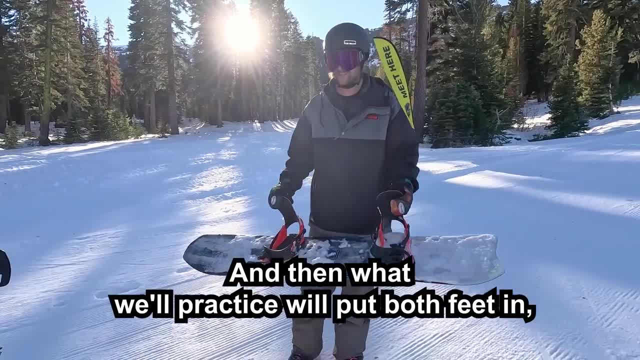 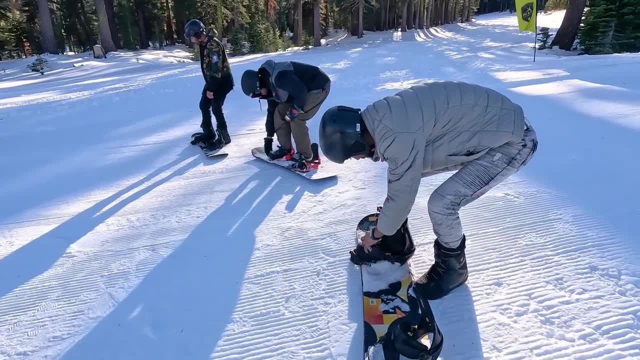 one hand on it and then what we'll practice? we'll put both feet in and we'll just practice like sliding down on this, like heel edge- Yeah, You're going to use a lot of force on your feet. Yeah, You're going to use a lot of force on your feet. 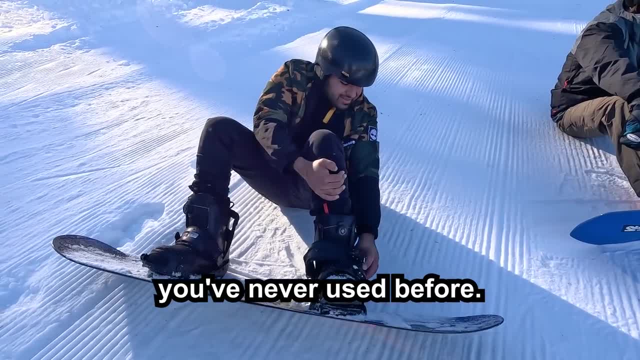 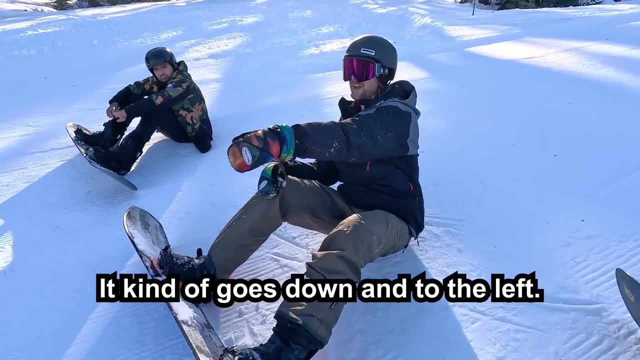 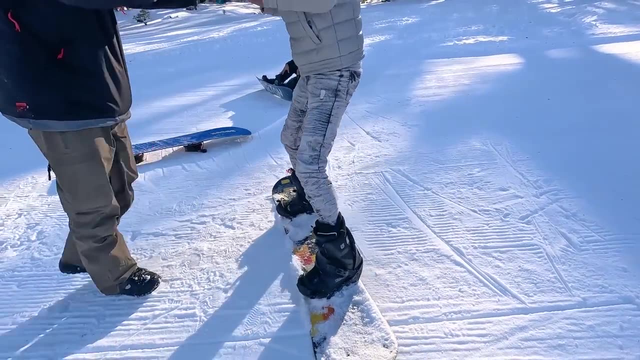 Yeah, You're going to use muscles you've never used before. So one thing to be aware of is where the hill goes. It kind of goes down and to the left, So we're going to go that way, Yeah, so lift up your toes. 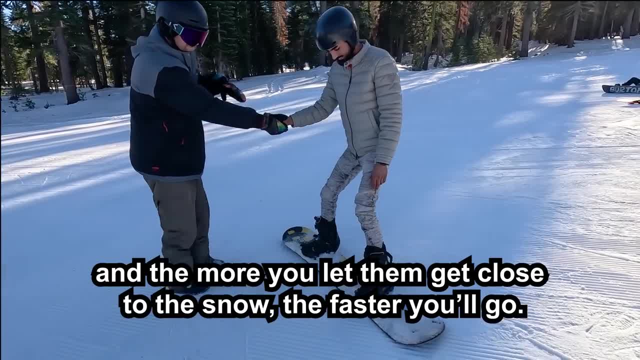 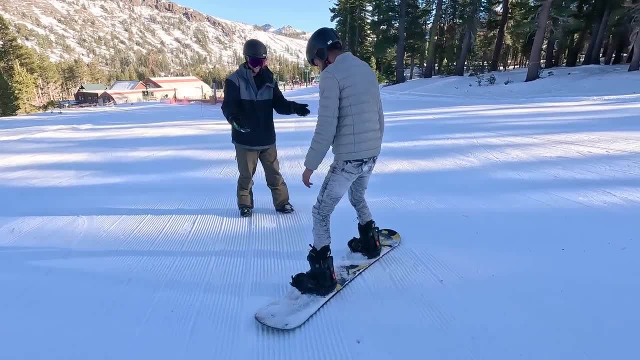 Yeah, the more you lift your toes up, the slower, and the more you let them get closer The snow, the faster you get. Yeah, nice man. So this is called the heel sliding. It's your turn, Zee. it's your turn. 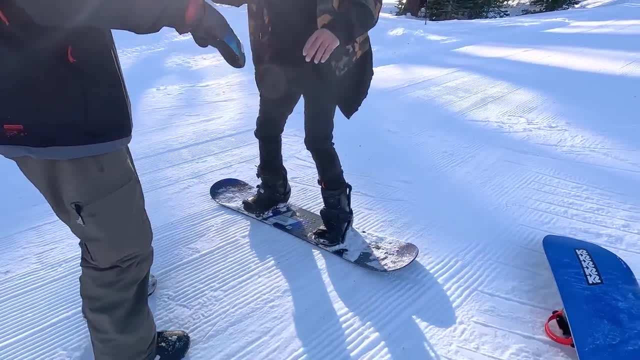 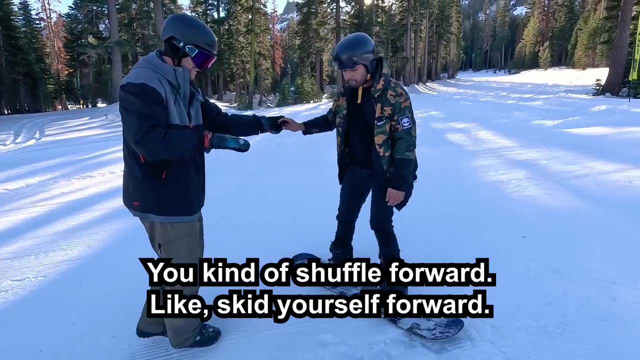 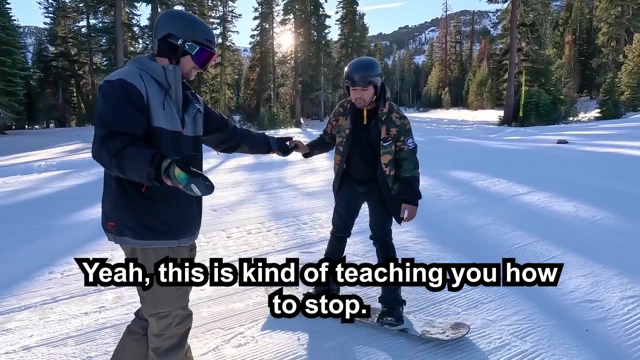 Let's do it. It's kind of like a shuffle, so you're just like lifting your toes up a little bit so you kind of shuffle forward, like skid yourself forward. Yeah, this is kind of teaching you how to stop on that. This is what hit me up last night, a little bit scared, but I was like, are you sure? 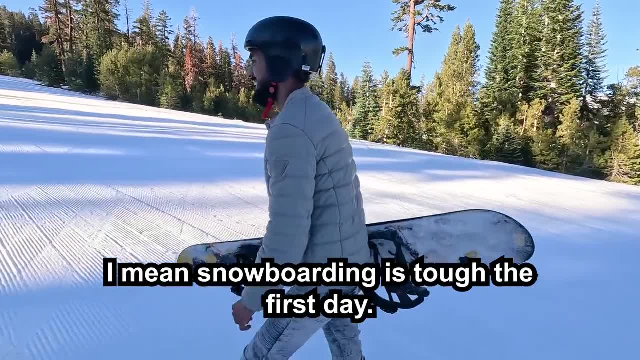 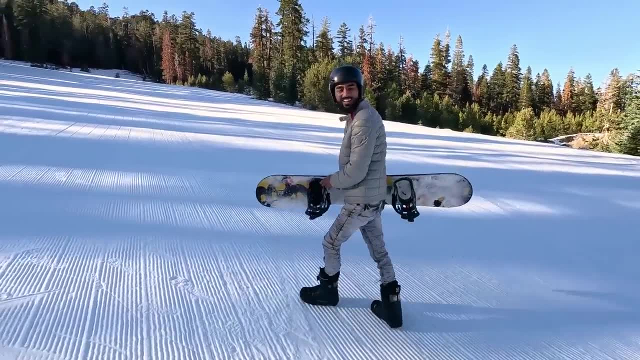 Yeah, I'm like: okay, let's go. I mean, snowboarding is, let's say, tough the first day, Don't worry, skydiving is next. man, I'm not doing it. After you guys can do the heels, the next thing to learn would be to slide backwards on your toes. 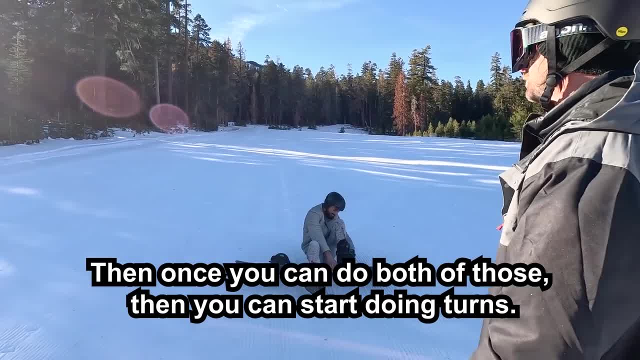 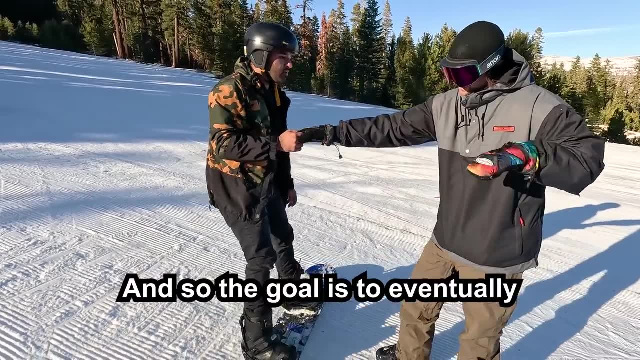 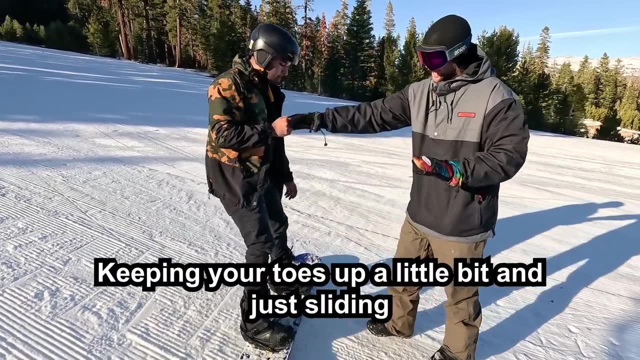 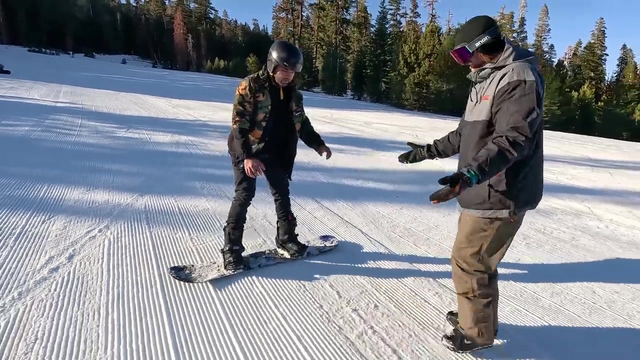 And then, once you can do both of those, then you can start doing turns, And so the goal is to eventually just slide smoothly on your heels, So keeping your toes up a little bit and just sliding smoothly the whole way. That's it, man. 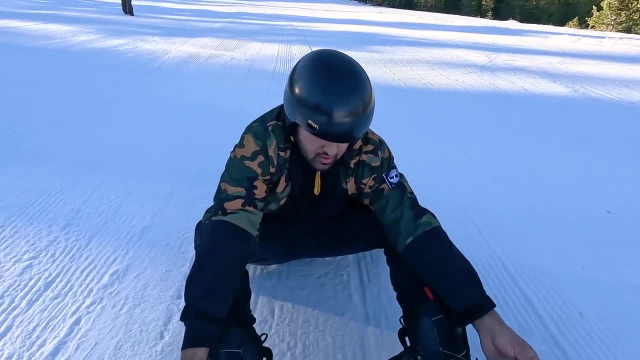 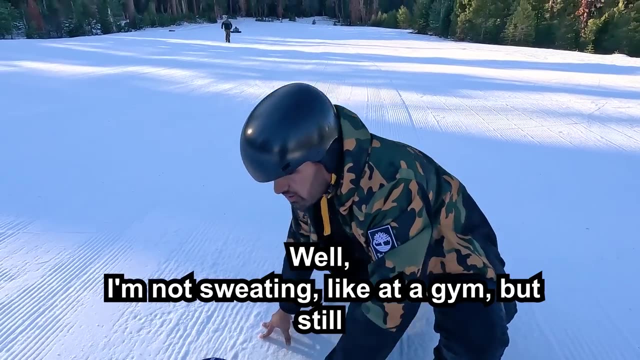 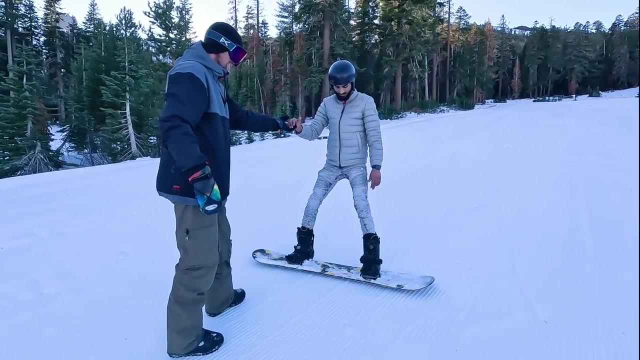 Nice man, How did that feel Good. actually, One thing: I didn't think you'd be that much of a workout. Well, I'm not sweating like at a gym, but still you get tired. So whoever set up this dance, it's too wide. 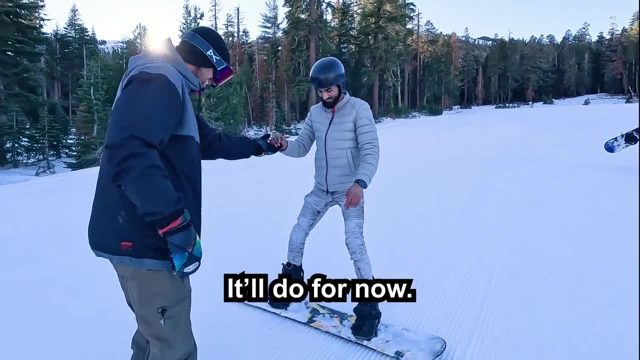 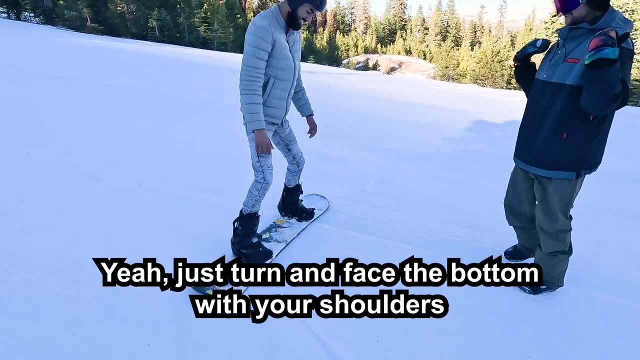 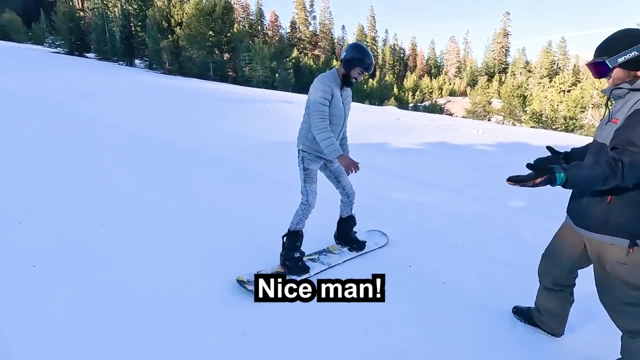 I can do that. It'll do for now, Even if you're good. yeah, just turn, Face the bottom with your shoulders. Your board will follow where your shoulders are facing. Nice man, How's your hands? Do you want some mittens? 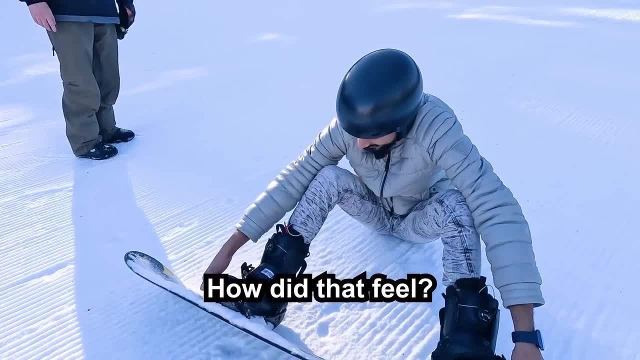 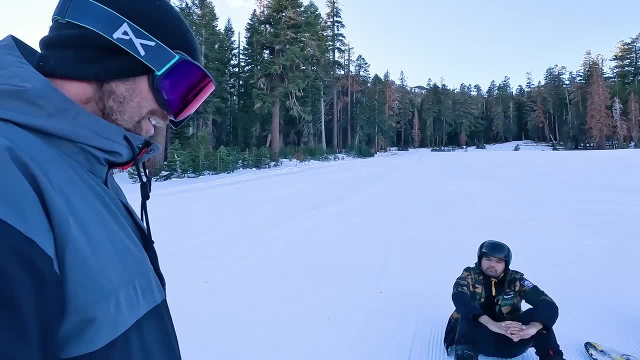 I'm cool right now. You're okay. Yeah, they're not that cold. How did that feel? It feels good, honestly Awesome. It feels good Like you're learning more. you know Getting there. You guys want to try sliding on your toes. 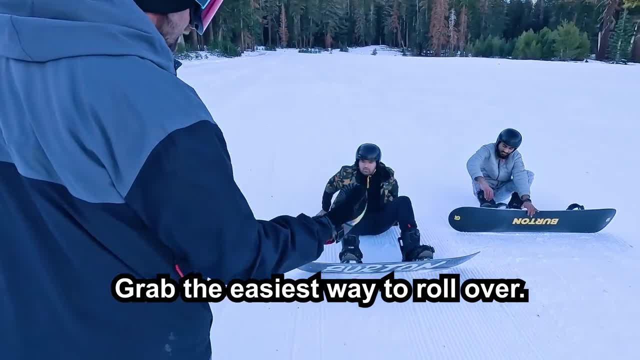 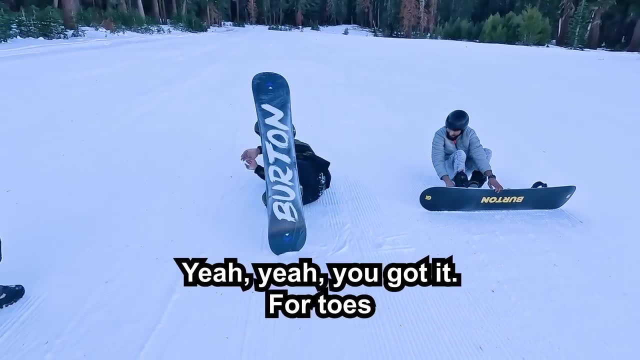 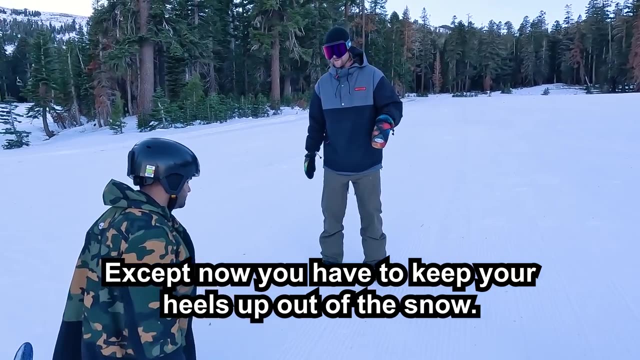 Yeah, So if you can roll over, So grab the easiest way to roll over: grab one knee and pull it over. Yeah, yeah, you got it For toes. it's like the same thing, except now you just have to keep your heels up out of the snow. 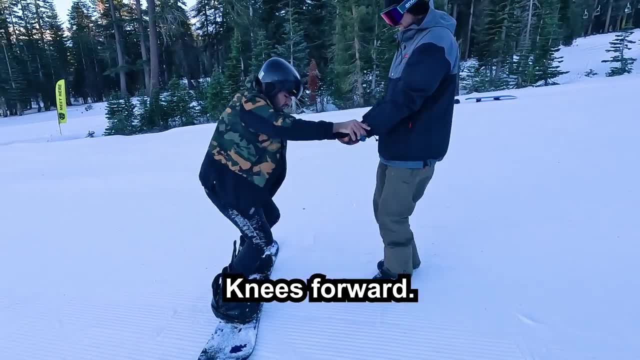 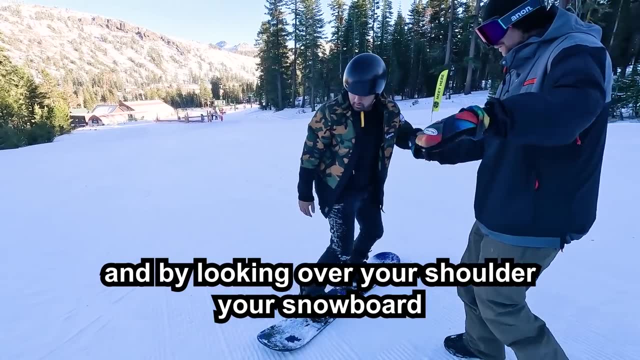 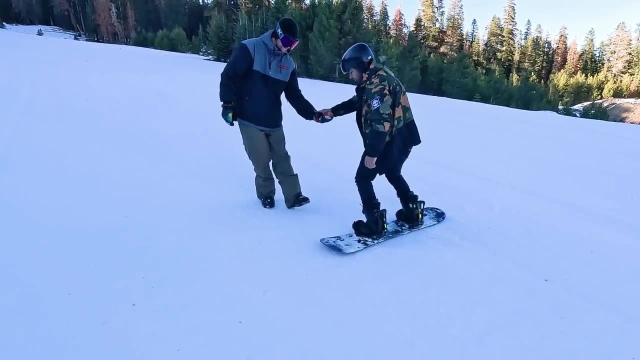 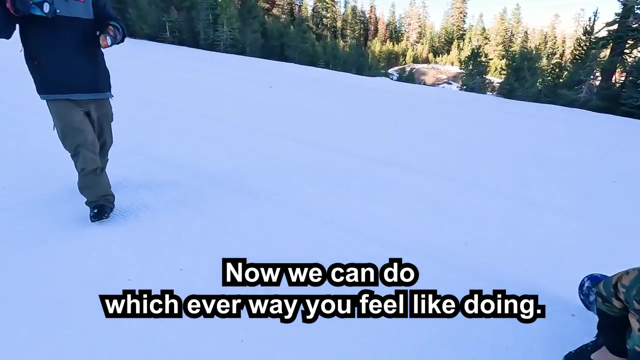 Yep, that's it, man. Like knees forward. Yeah, Just keep those heels up. And by looking over your shoulder, your snowboard will naturally want to go that way, Just like by looking this way. So now we can do whichever way you feel like doing. 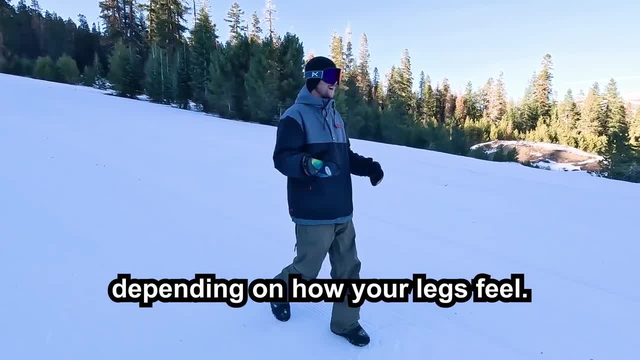 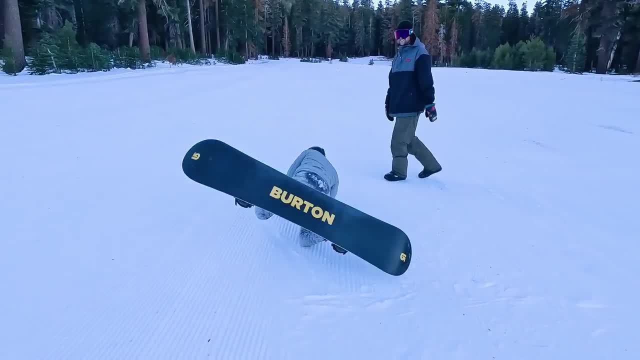 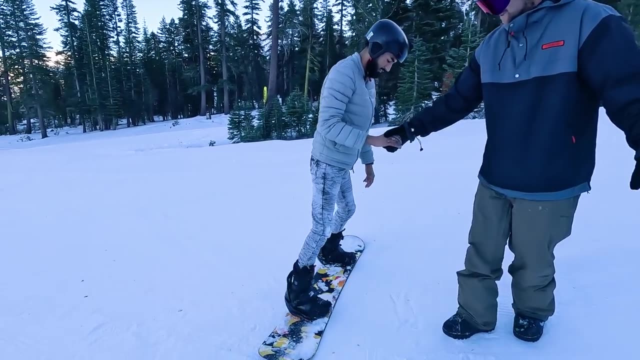 You can slide on the heels or toes, depending on how your legs feel. Let's get Ali to try his toes Shuffling backwards A little shuffle and just keep those heels. Yeah, bending your knees forward? Perfect. Let's try to go all the way across. 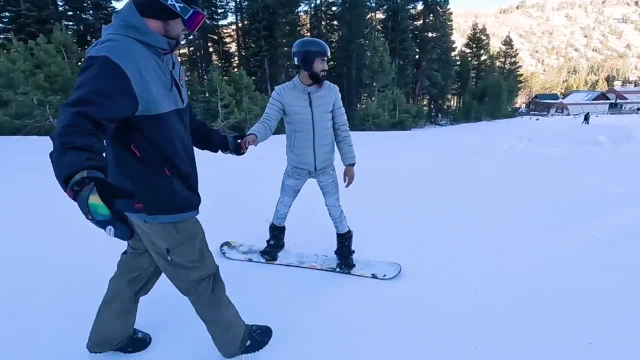 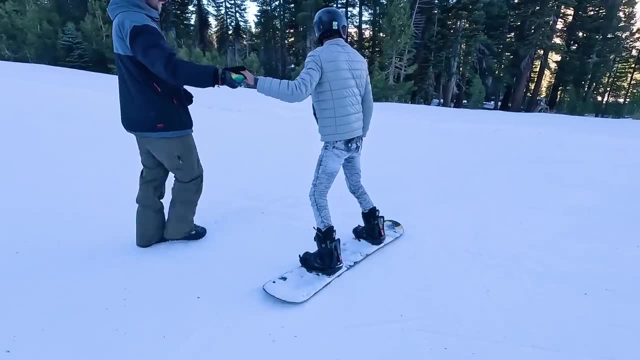 Yeah, whatever way you look is the way that you're doing. You're very close to doing what my legs are doing. You're killing it. Yeah, just knees forward And then face your chest to the bottom And then your heels. 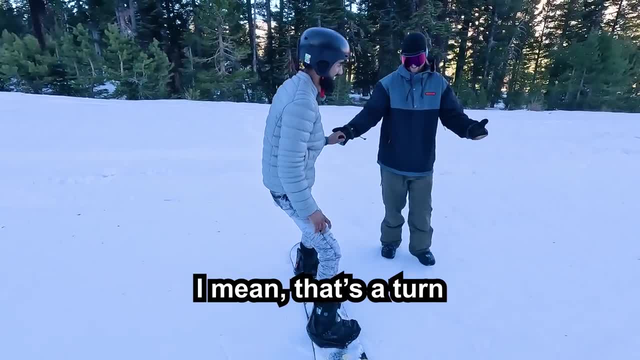 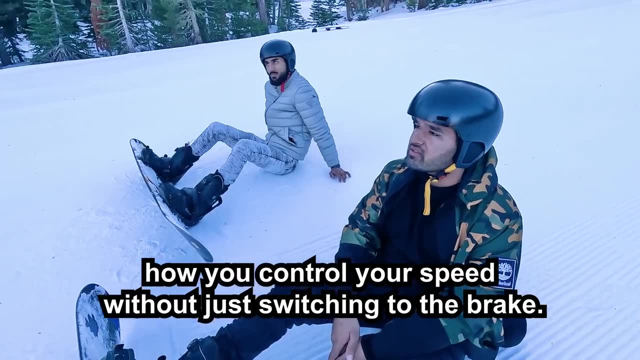 Yes, that's it. Cool, I mean, that's the turn. Wait. so if you're going down, how you control your speed without just switching to the brakes? So right now we've been practicing the heels, right, Yep. 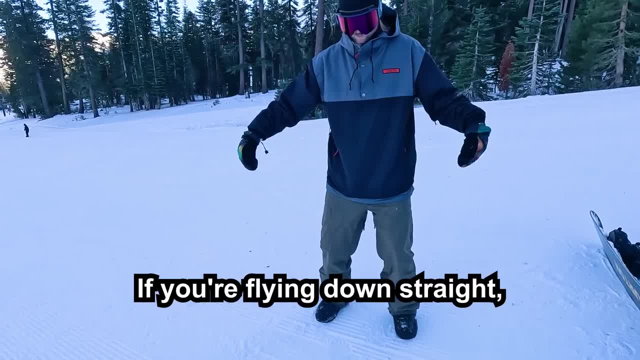 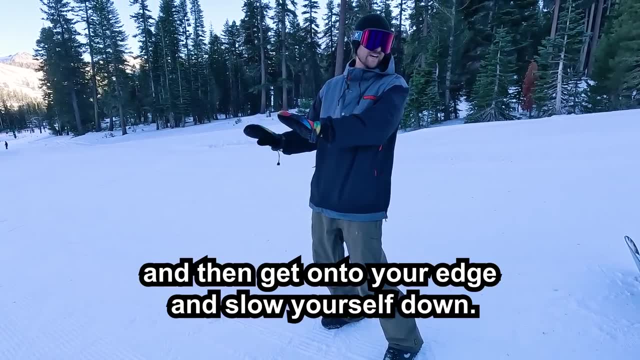 And did some toes. So if you're flying down straight, what eventually will happen is you'll be able to turn yourself and then get onto your edge and slow yourself down. So that's what we're learning to do right now is to use our edge to like go slowly. 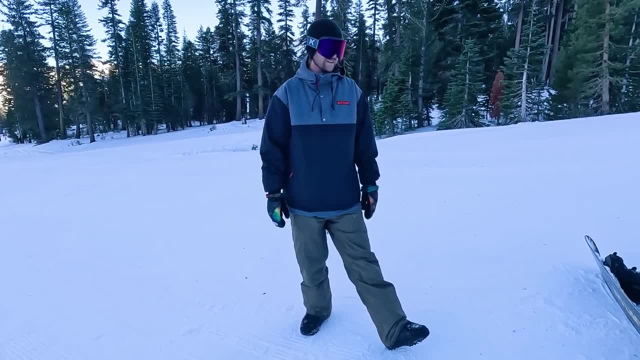 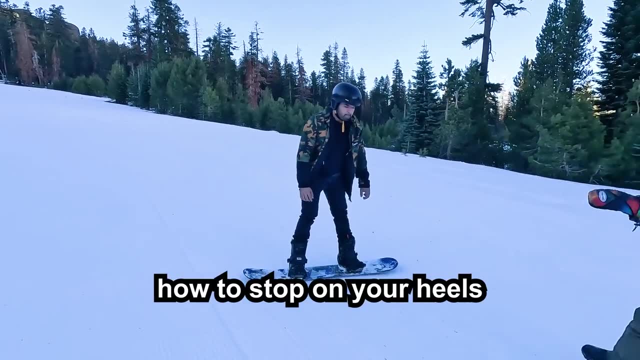 Oh, I get it now. So you guys are like We're like learning to stop, like right now, We're learning to stop, basically right now. Yeah, so this is teaching you how to stop on your heels. He's going for it. 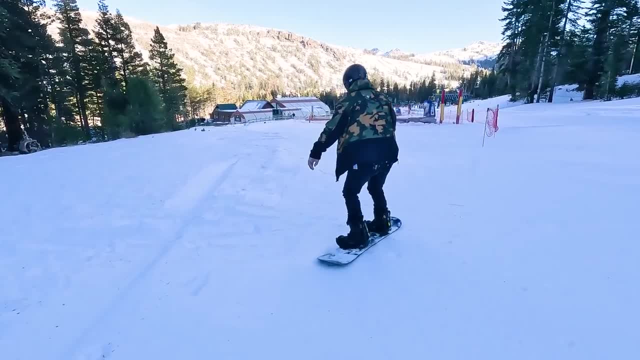 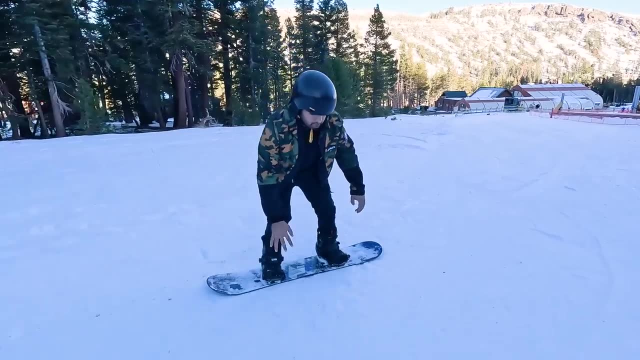 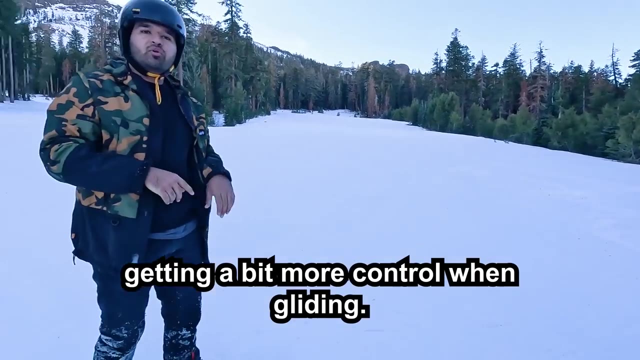 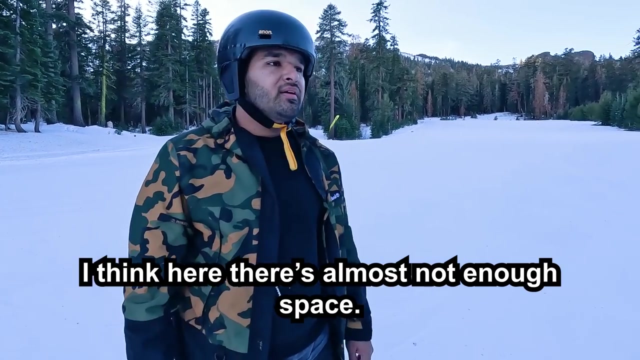 He's going. I got to practice my heel more. I thought I would have stopped- Yeah, Getting a bit more control when gliding, But there was a really loose snow there so I kept dragging that way. I think here it's like there's almost like there's more, not enough space. 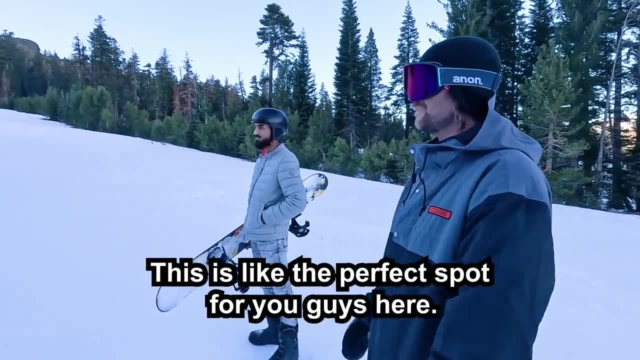 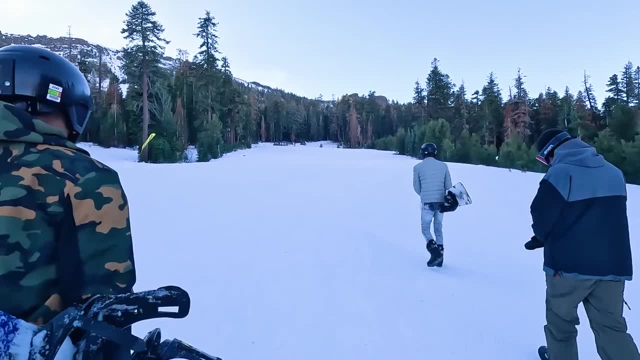 Yeah, Up here it's just like so wide. This is like the perfect spot for you guys. Yeah, Dude, do you need some? Do you want some mitts? No, it's good. Oh, okay, Once you're comfortable on both, then you can actually go from your toes onto your heels. 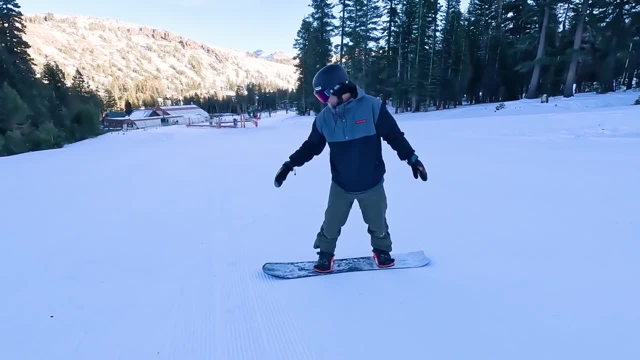 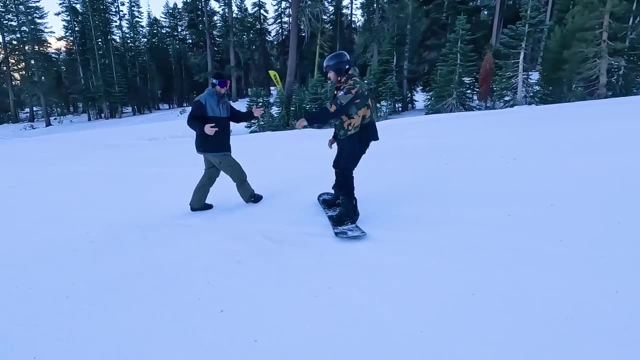 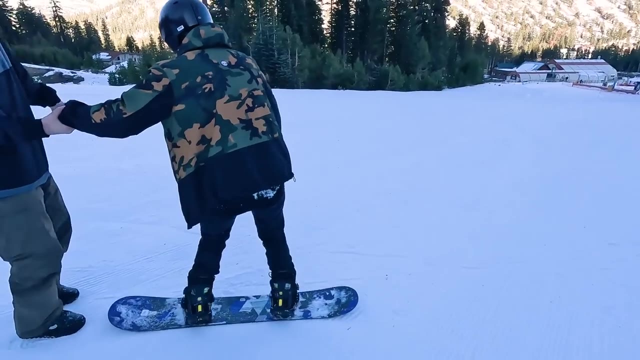 Like sliding. Yeah, I can actually help you as well. Go straight, Yeah, So go straight. and then toes Nice, And then, when you're ready, straight, Have you one more time. Yeah, Yeah, That's good Yeah. 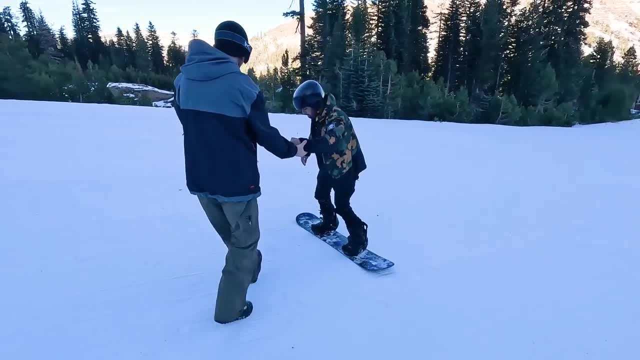 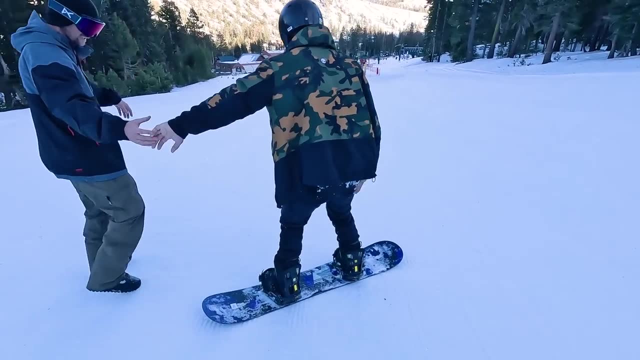 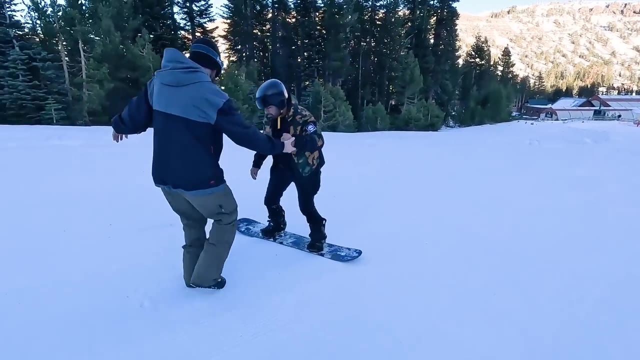 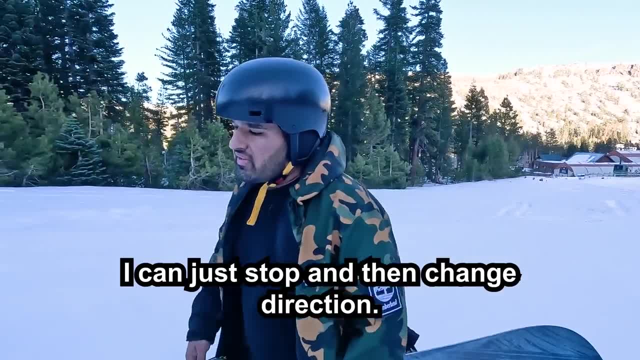 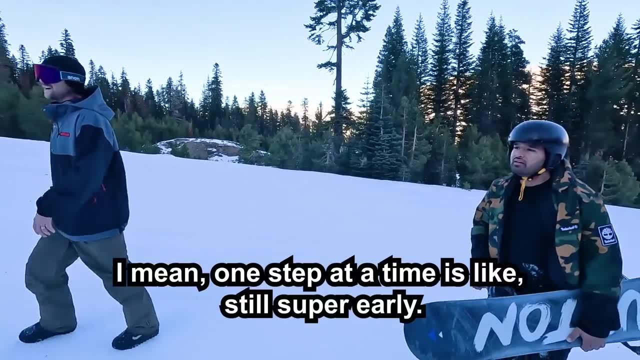 start to pick up speed. I can just stop and then change direction, But with toes still having a hard time, just stopping Toes is harder for sure. Yeah, But yeah, I mean one step at a time. it's still like super early. 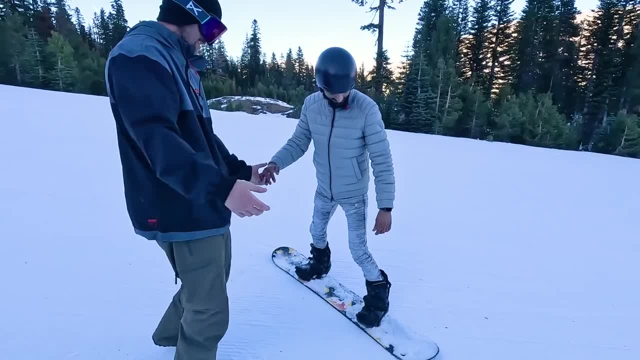 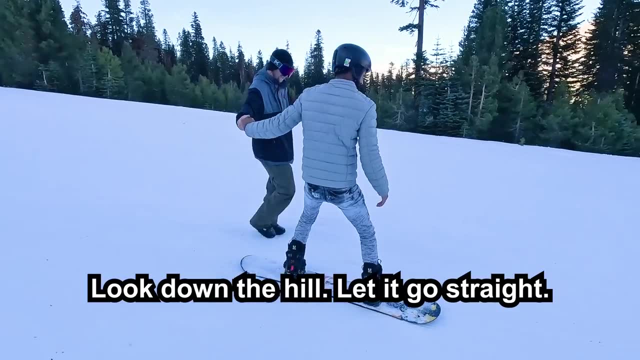 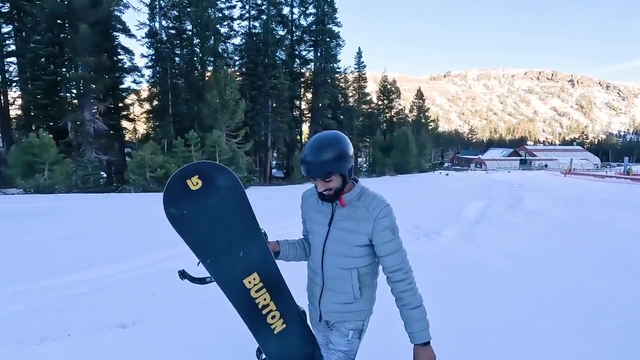 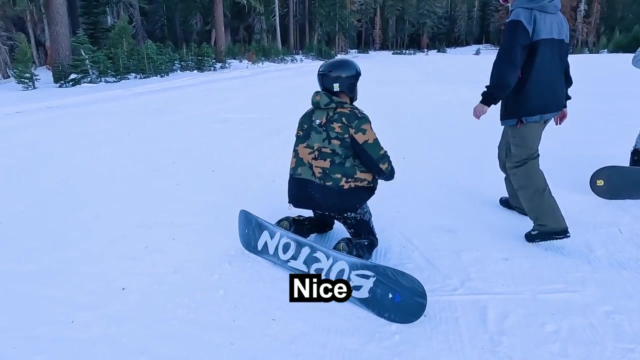 Is the toe starting to get a bit easier? Uh-huh, Uh. So look down the hill, let it go straight and then swing it to your left. Awesome, there, It's getting colder and colder. Nice, You're going to use that other hand. 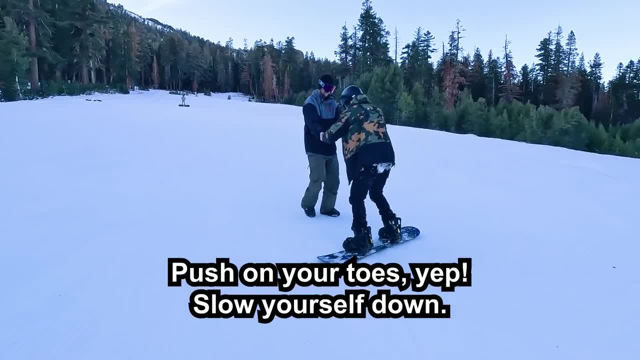 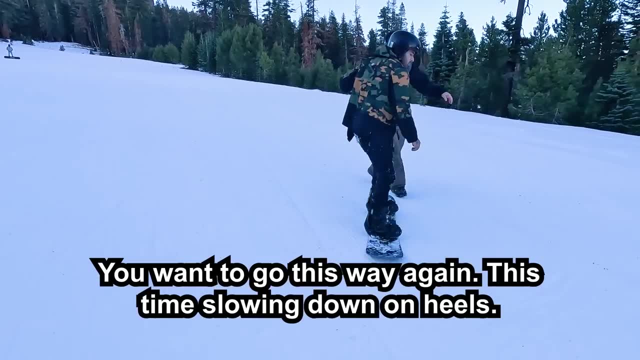 Push on the toes, Yep, Awesome. And then again back to the right side. So you're going to go this way again, Yep, And this time stay on your heels, And then, Oh no, go right foot again. 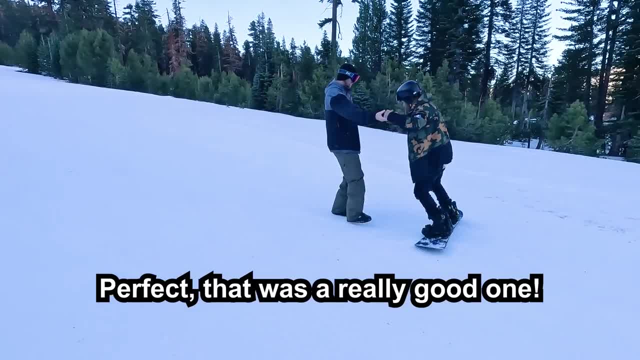 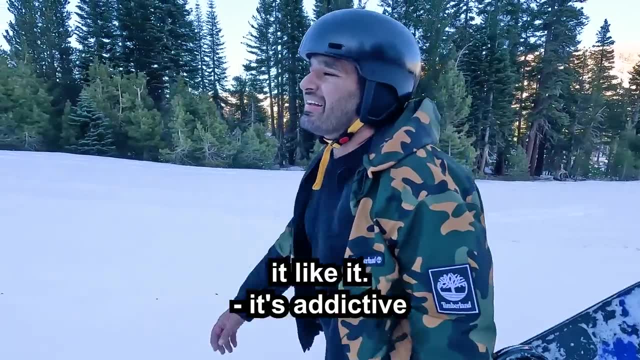 Yep, there you go. You know it's tiring and keep messing around, but I don't want to stop. It's addictive. Oh yeah, Man, I've been wanting to do this sort of thing for a long time, but it scared me too. 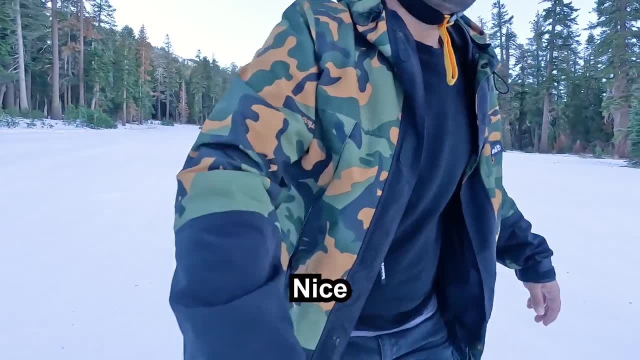 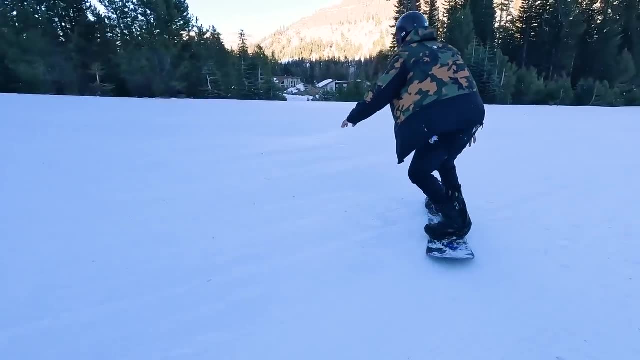 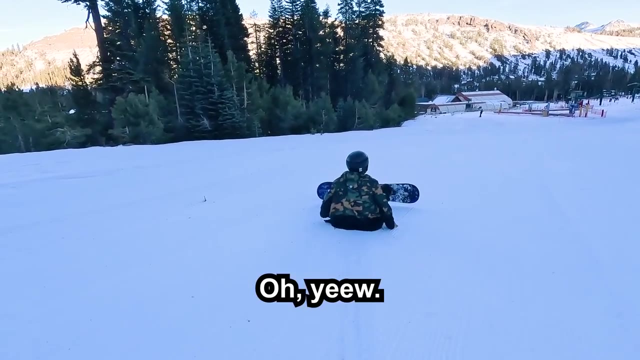 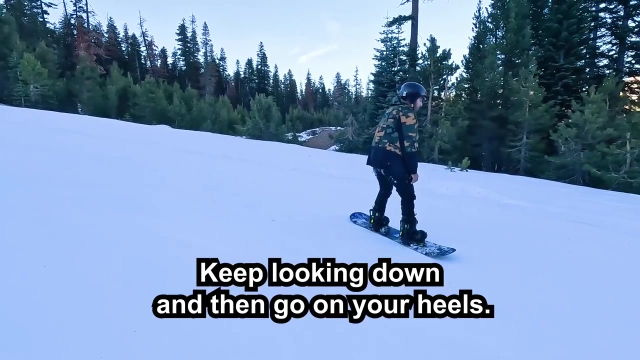 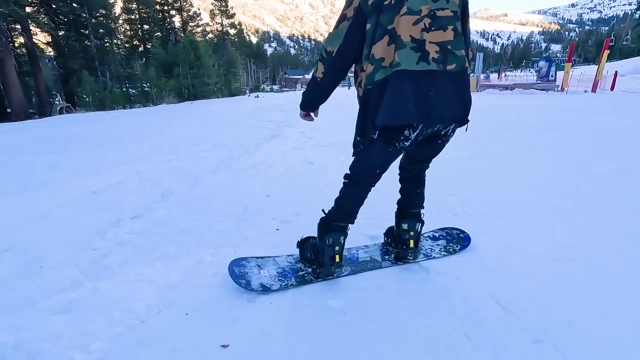 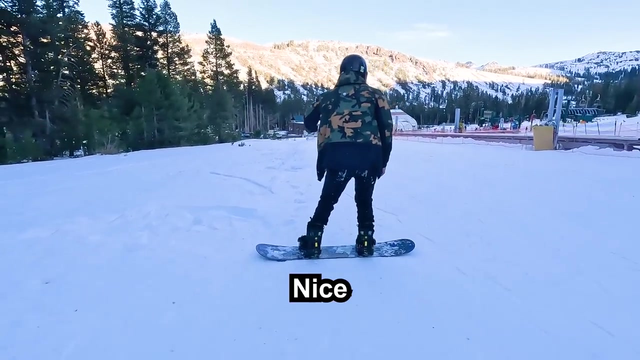 You know, you got to try it. Nice, Slow, slow, Yep, Yep, nice. Keep looking down and then go on your heels. Heels, heels, heels. Yes, Nice, Are these your guys' mitts? 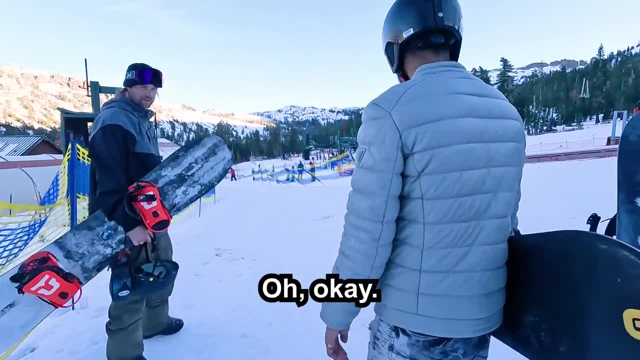 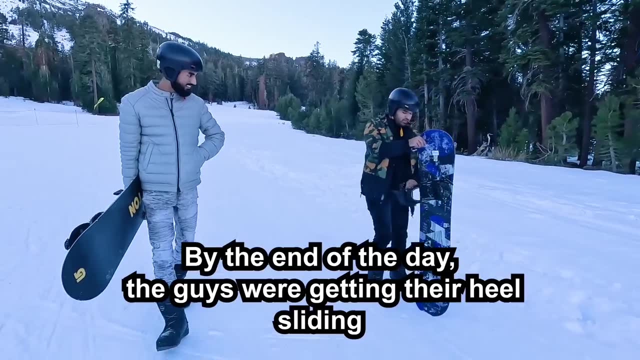 Oh, no, We didn't bring any. No, We didn't bring any. Oh sweet, Okay, All right, You guys are snowboarders now Tired of it. So by the end of the day, the guys were getting their heels sliding and toes sliding down.